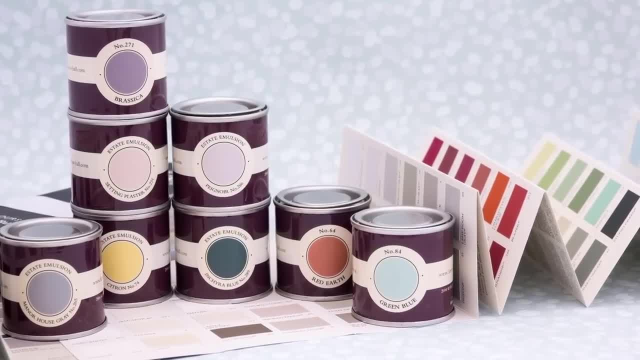 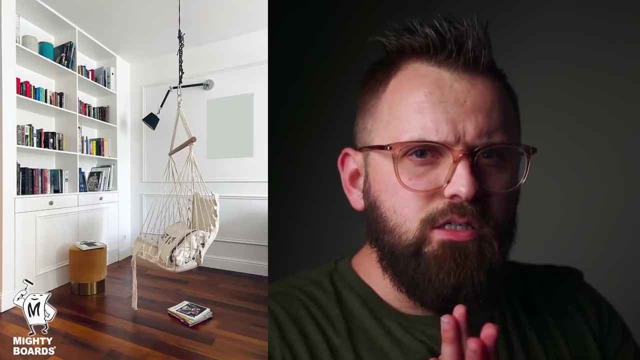 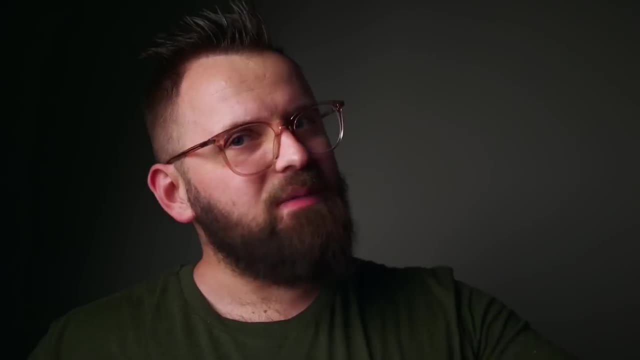 order little tester pots which you can then paint onto a tester board like a Mighty Board, which is our favorite tester boards. But just double check, though, that when you're ordering testers from Farrow and Ball, you're actually getting the paint can like the actual tester pot, because I've seen people 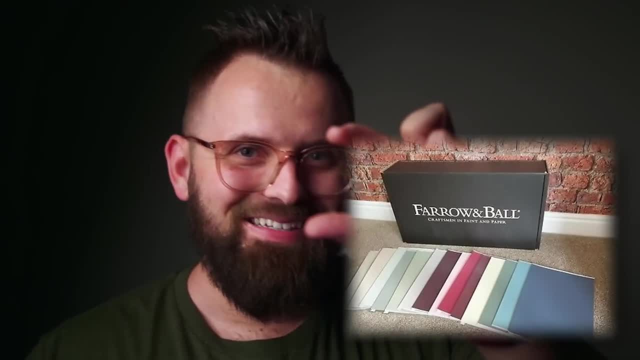 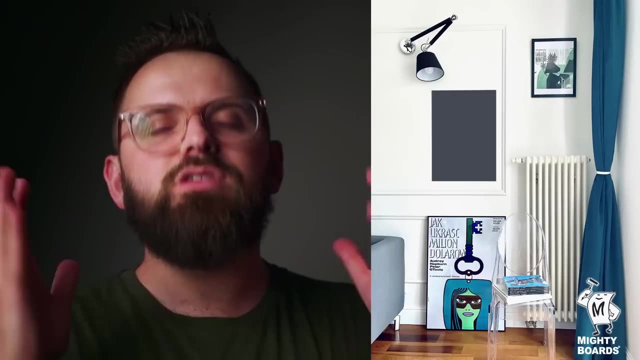 online complaining that they just get sent a little tiny swatch instead. And also, if you don't know what Mighty Boards are, then you must be new to the channel, because we love them. They're large, flexible. You can use the same tester board in multiple rooms rather than just limiting. 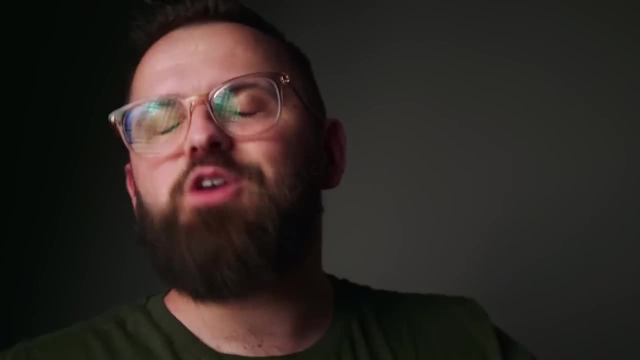 yourself to something you painted on a wall. Their information, as always, is down below in the description, so you can check it out And, if you're interested in learning more about them, check them out afterwards if you want to pick some up. 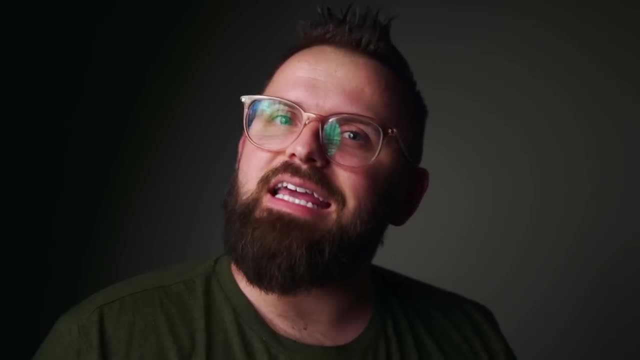 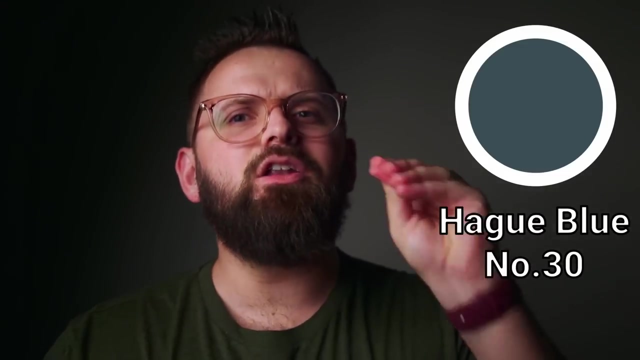 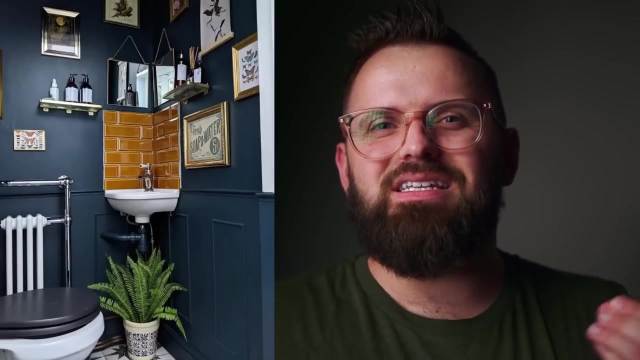 Anyway, let's get into the colors. The first one we're going to look at is Haig Blue, And although I could have gone for a variety of navy blues, Haig Blue is definitely a notable one. It's extremely rich, like most navies, but there's something about it that really feels dynamic. 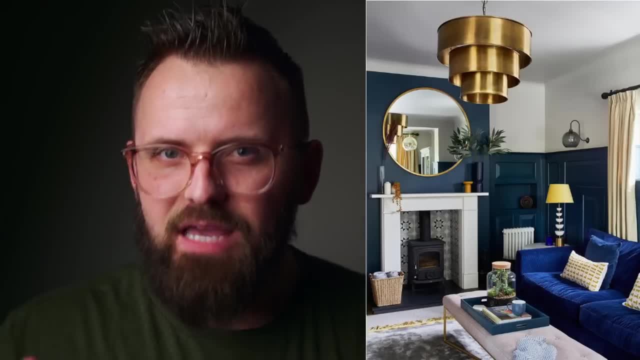 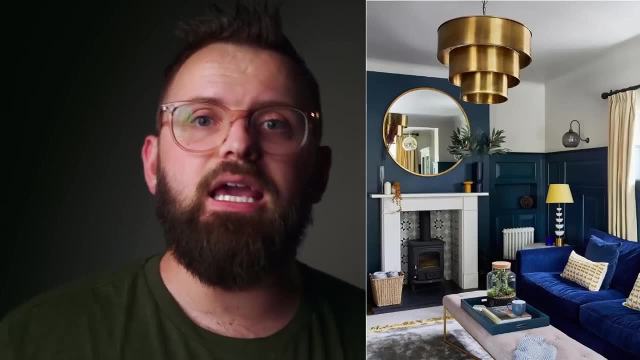 and captivating. In the world of navy blue, I would say. this color has just a touch of teal that may or may not show up in your home, depending on your lighting. So if you're into lighting and, I guess, any surrounding colors that you have or like to incorporate, So it has. 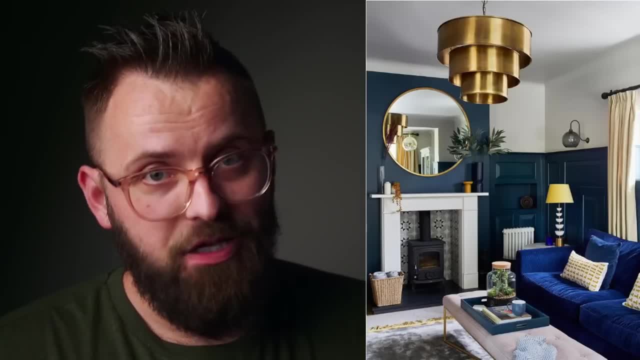 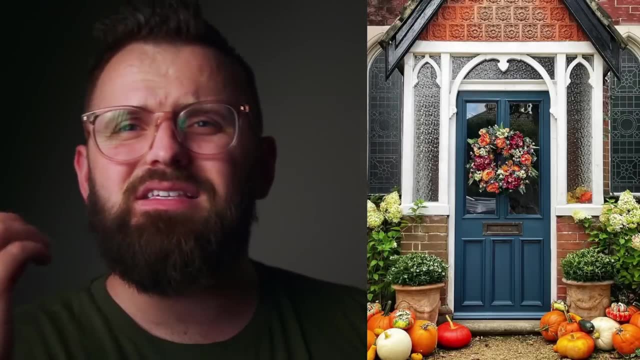 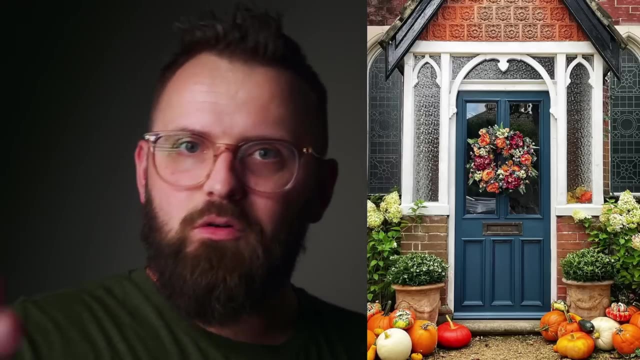 that little bit of nuance that makes it really, really interesting and quite gorgeous. I obviously picked a Farrow & Ball navy because their colors are so deep and saturated And, fun fact, they're actually pre-made in a factory, So you're not going to find at your local Farrow & Ball paint. 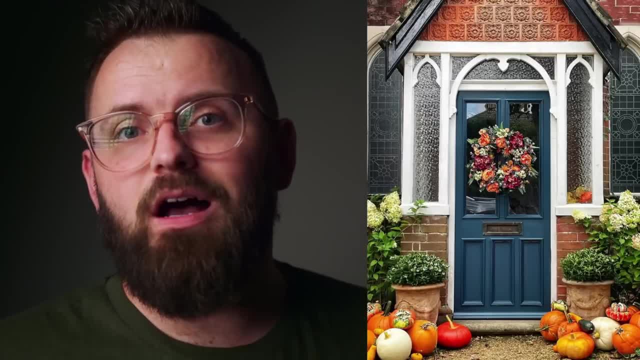 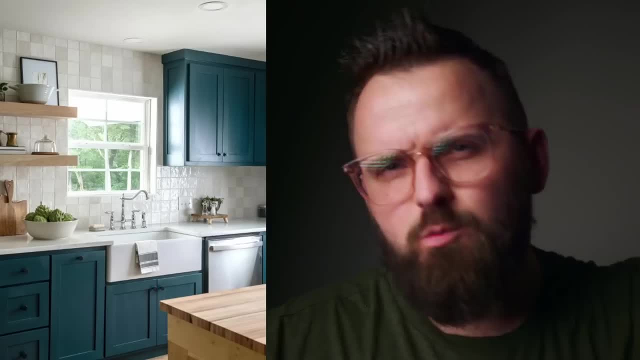 store anyone mixing or tinting cans. like everywhere else, They all come pre-mixed and just a quick shake and then you're done. I wonder how they get all that color in there. Haig Blue is a gorgeous wall color for the more secondary spaces in your home. You could also use a color like this. 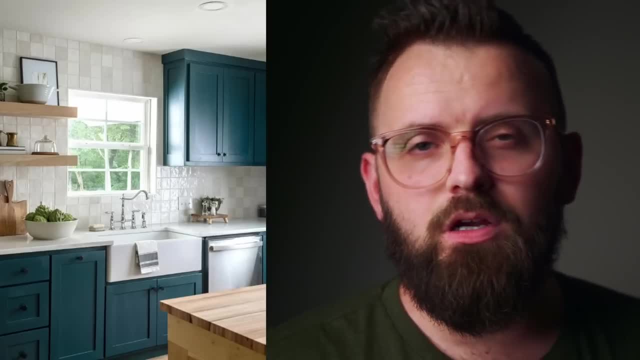 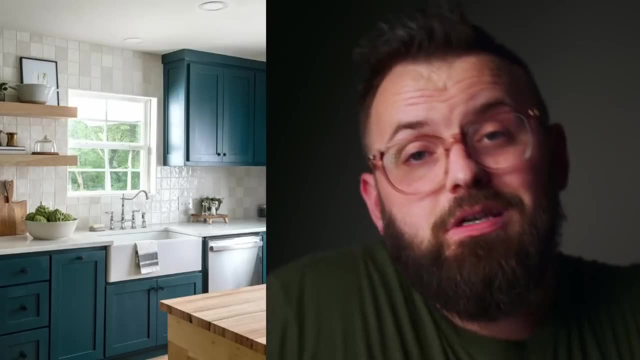 on your kitchen cabinets, which is still very popular, And I can't really see it going out of style anytime soon. really Maybe a bit repetitive, but it works, So you can't really argue with that. This color is beautiful. The next one we got to talk about is called Railings. 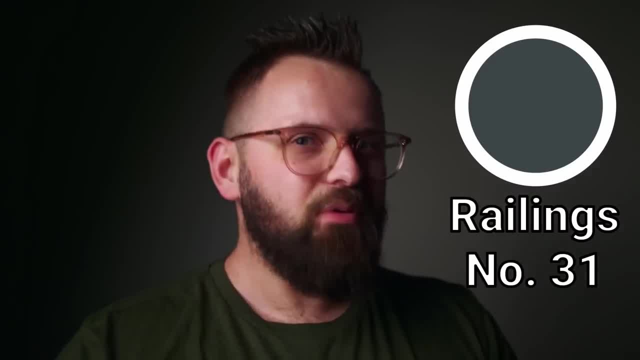 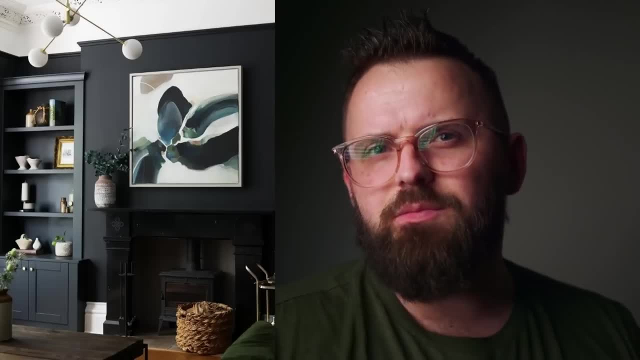 which is a bit of an off black by Farrow & Ball, And I find that black never really goes out of style, right. But off black shares that quality as well, and it gives you a little more flexibility too, Because sometimes you're looking for a black that is just a bit softer. which Railings is It's? 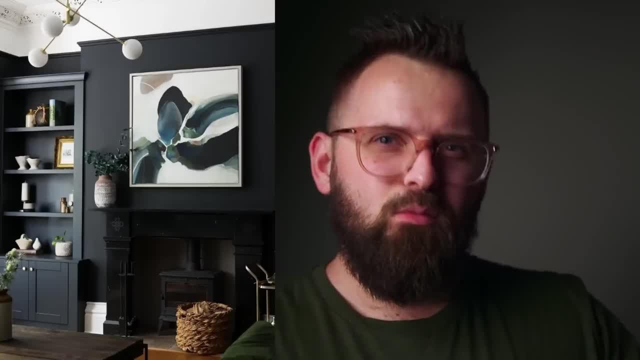 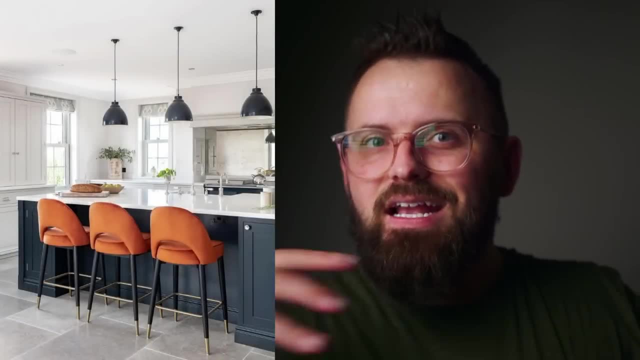 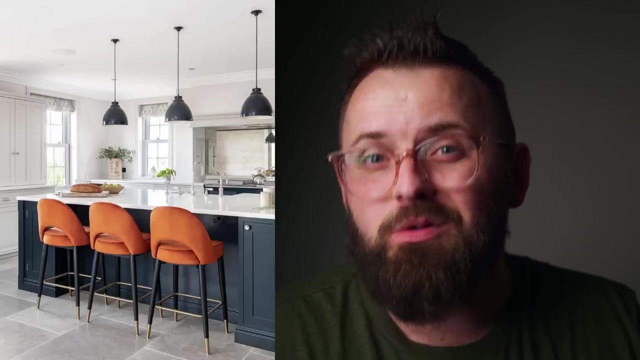 also ever so slightly cooler as a black, which tends to be more commonplace with all black paint colors in general, And the reason for that is if you have a warmer black, it ends up going into almost espresso brown territory or even slightly earthy kind of greeny territory. 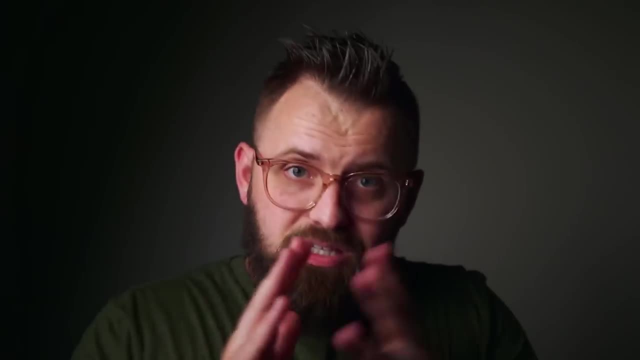 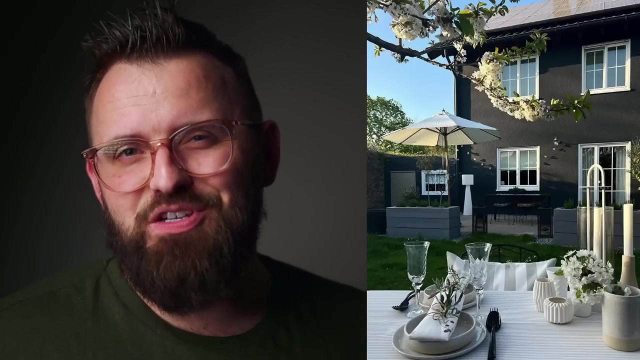 it could go against certain color schemes, But Railings doesn't really do that. It doesn't have that problem. It's also not the darkest black paint color that exists, but it's one of my favorites, especially within Farrow & Ball. No one's going to get sick of this, unless you maybe paint your. 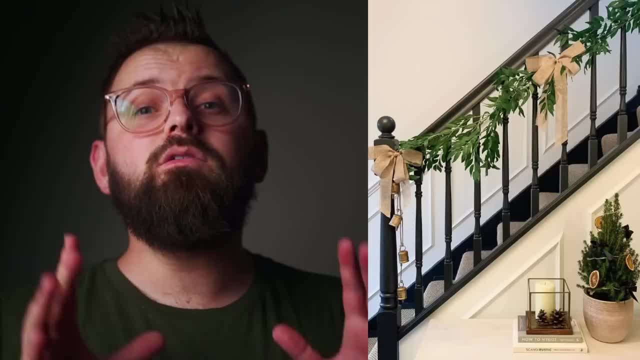 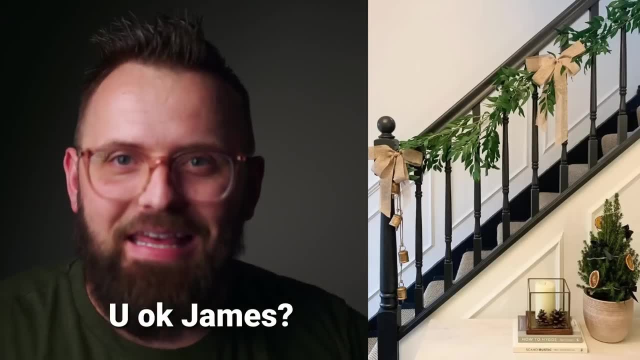 entire kitchen with it. Then that might get a little old One. very popular use case for using a color like Railings is to paint your railings with it right, So funny. But also as an opposite alternative to white trim and woodwork, which is a little bit more commonplace with black paint. 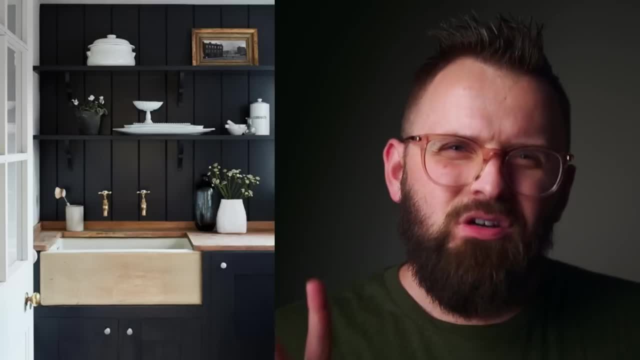 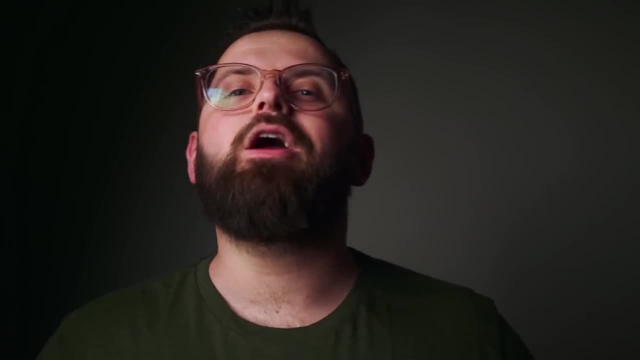 where you could theoretically use it on your baseboards and your frames, but more so, I see it as a fantastic door color choice, both inside and out. Now that we got the uber saturated Farrow & Ball colors out of the way, let's flip the script and opt for something much lighter that. 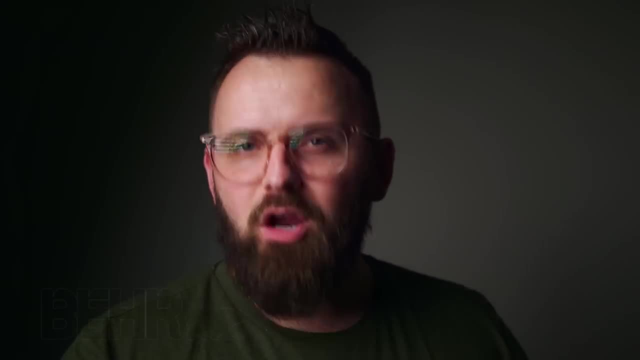 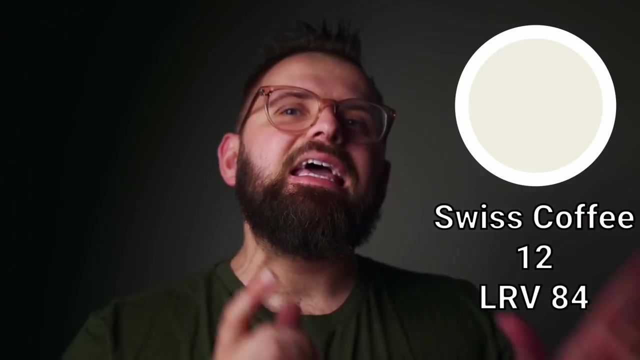 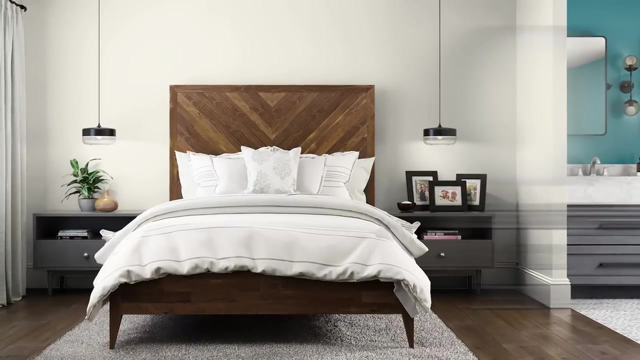 you'll probably see more often inside your home. Starting with Behr Paints Swiss Coffee, This color is part of the white color family, but more specifically it's an off-white that has this white chocolate Creamy warmth to it that makes it very comforting and inviting All colors in general, they can lean. 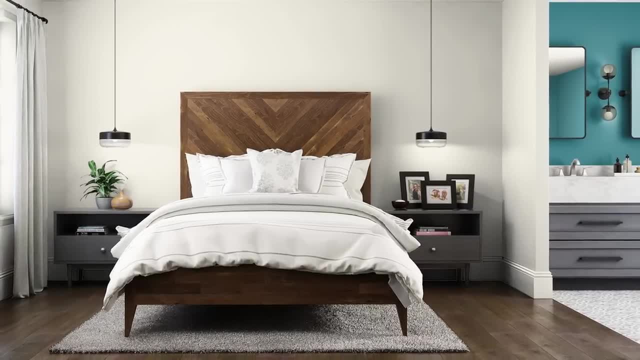 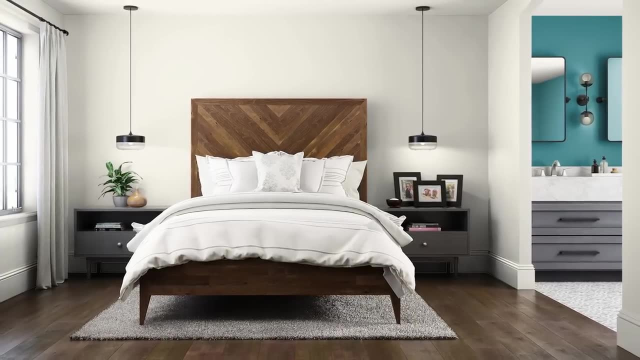 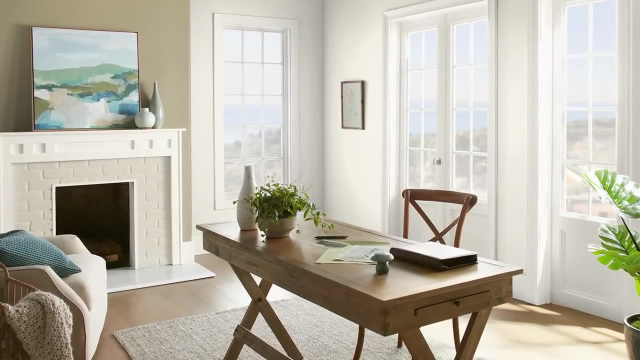 warm or cool, and this is especially important to decipher when talking about off-whites, because a cool white could look quite literally icy and frigid and very stark and sterile, while something like Swiss Coffee brings in that cozy warmth that is perfect for inside the home, That yellow within. 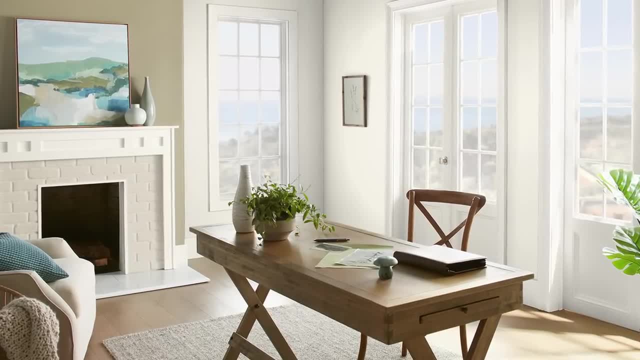 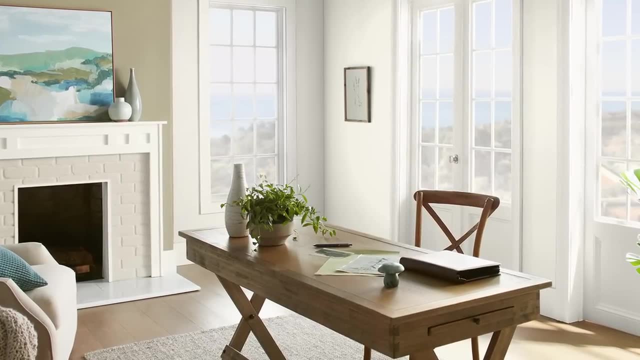 it is somewhat noticeable when you compare it to a brighter white, but it will seem much more subtle as a standalone color if you wanted to use it on your walls, for example. Little side note as well: Benjamin Moore makes a color called Swiss Coffee 2, and, believe it or not, there's some remarkable. 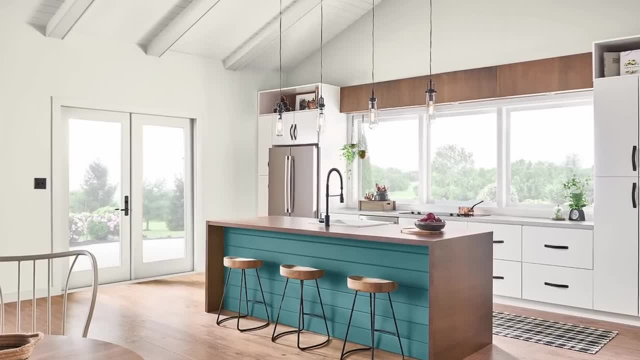 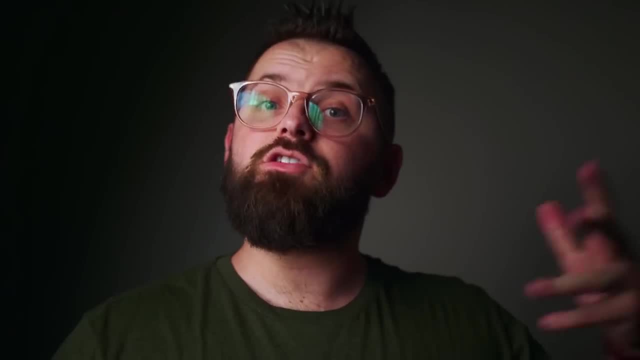 similarities between the two. I wouldn't say they're completely interchangeable. it's not exactly a perfect match, but they are certainly two peas in a pod- Off-white peas, not green ones- An alternative to Swiss Coffee that has a bit less of that creamy yellow warmth, or at least it's. 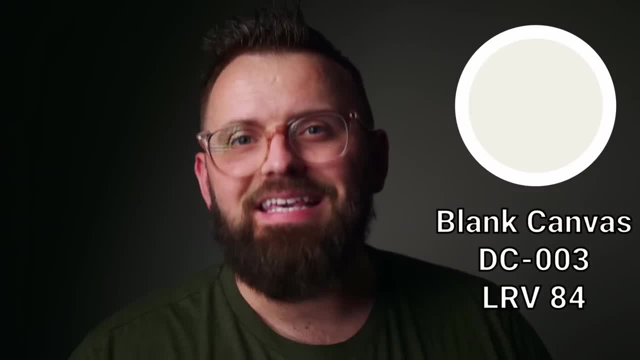 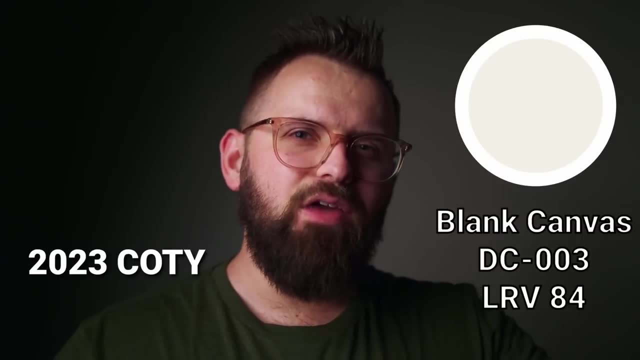 been toned down is a color called Blank Canvas, And this was conveniently Bare Paint's Color of the Year recently, and its name really gives away the reason why this is a timeless color: because it's the paint that you can use when you don't. 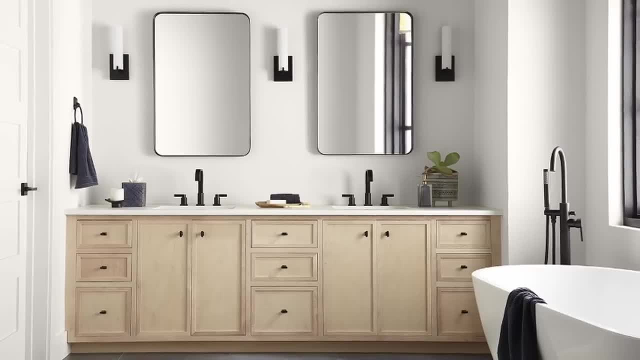 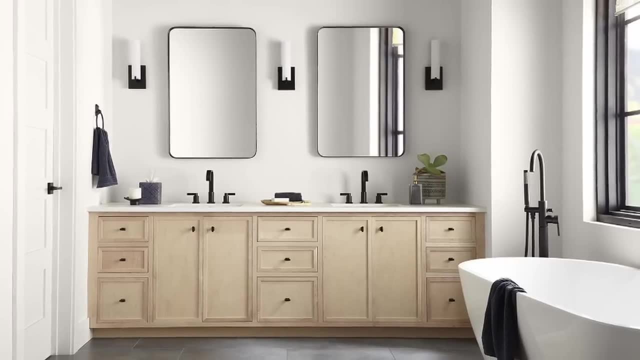 want your paint to really stand out, And that sounds kind of counterintuitive to people, but it is a thing. It's a clean slate color. If you're looking for something that can just blend in and remain light and airy, this is your choice. I think it's a more neutral choice than even a 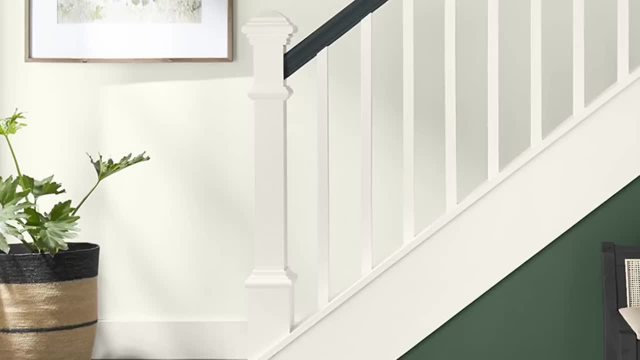 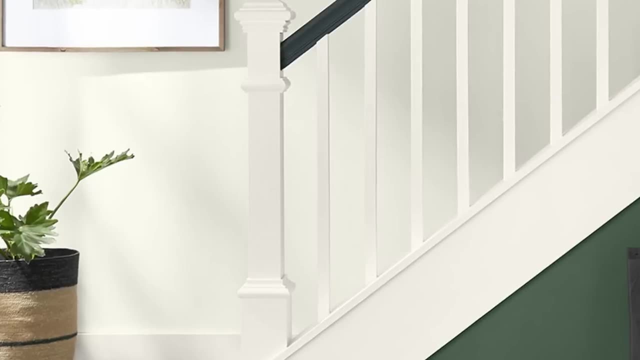 dark white, because those can go into cooler territory, which can throw things off. Blank Canvas allows you to put fun things on your walls and have them stand out, rather than the walls themselves, and I think that's why it was chosen. As we shift to Sherwin-Williams, which is our next, 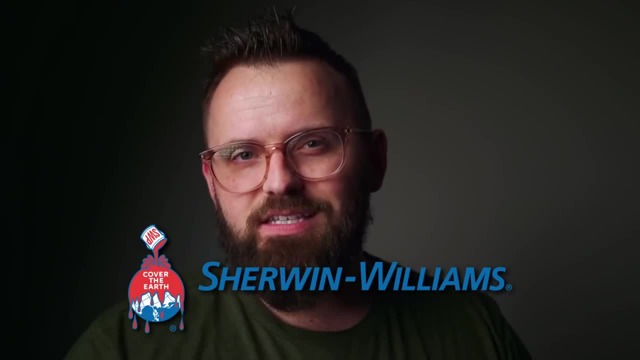 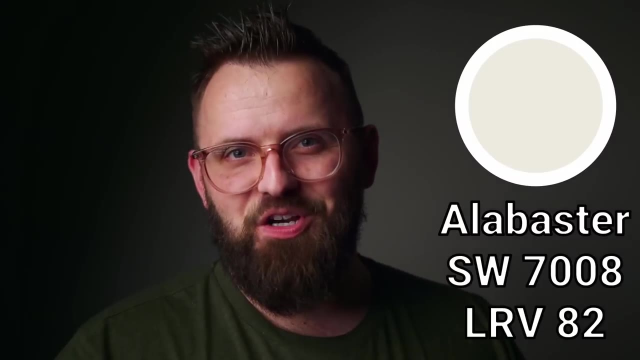 paint company. we have one of their mega popular off-whites that are even more grayed out than Blank Canvas, but only by a bit. It's called Alabaster and it is one of my favorite light neutrals to use If you're looking for a color that's a little bit lighter or a little bit more. 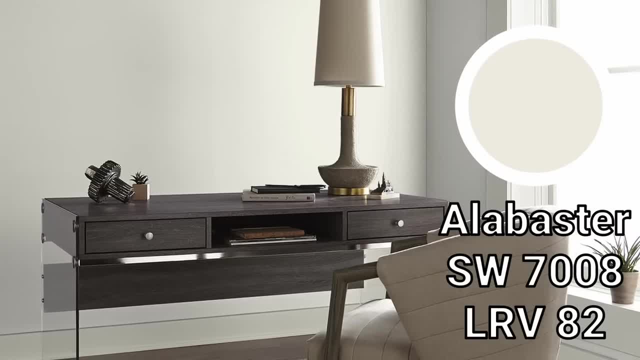 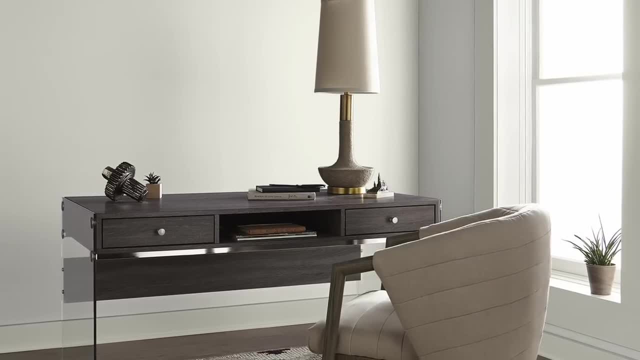 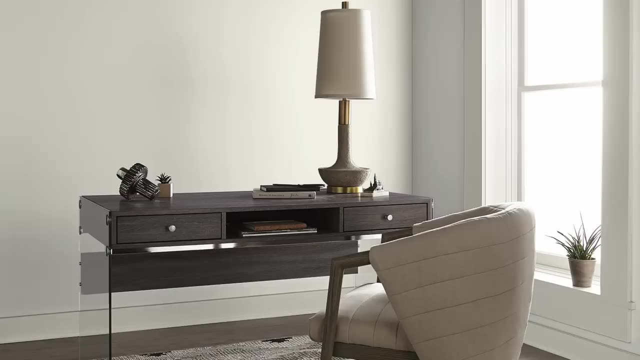 dark. it has such a wonderful balance of softness and some warmth, without feeling yellowy and dated. It just has this perfect combination that is very balanced and composed, and it also has just a touch more depth than the other two colors we just spoke about, So maybe you'll notice it a little. 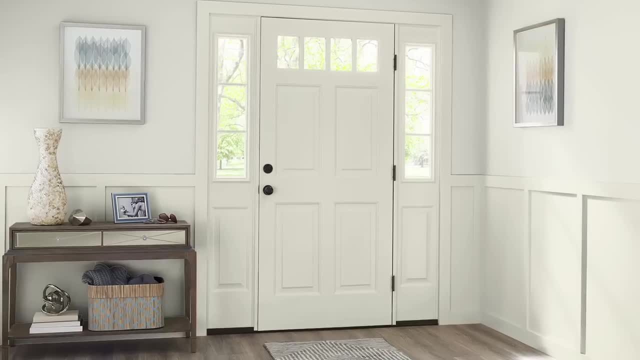 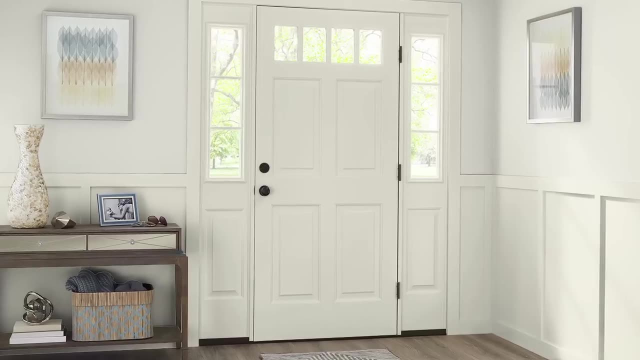 bit more, but not to the point where it's going to distract you. It's not going to pull focus or anything like that- And honestly I think it's a wonderful choice as a wall color, but you can use it as a more interesting alternative to pure white on your woodwork- Also a great exterior. 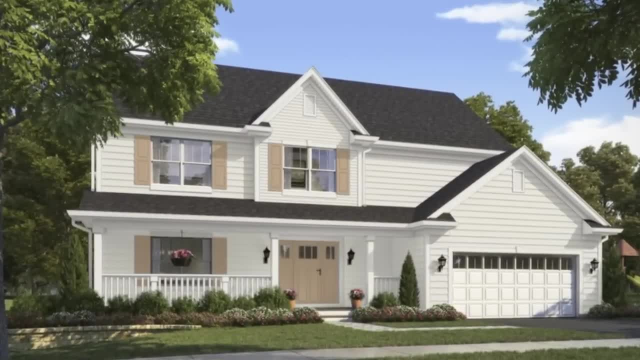 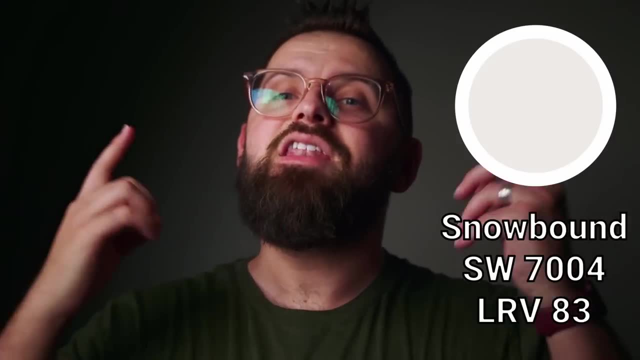 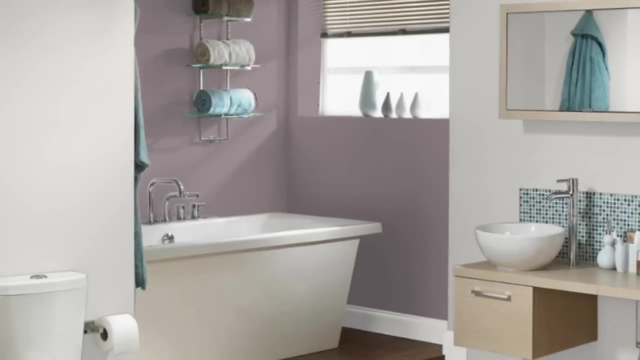 white paint color that you won't feel is too bright when the sun hits it. It's so balanced, so soft. I love Alabaster. Next we have Snowbound, which is another awesome off-white by Sherwin-Williams and I like to call it the taupey alternative to Alabaster. So the main difference between 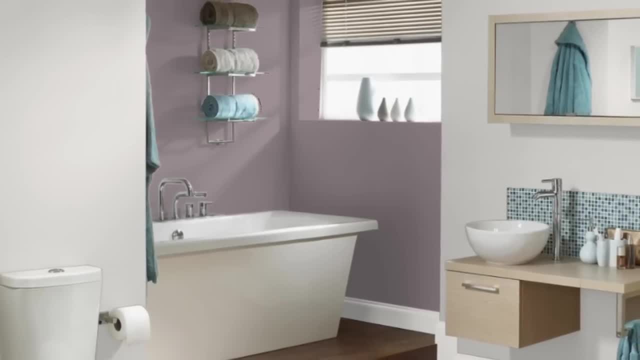 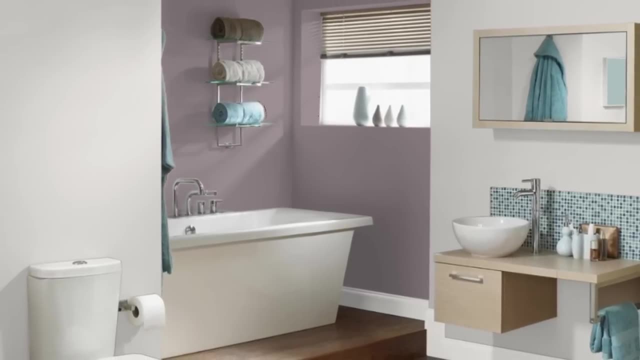 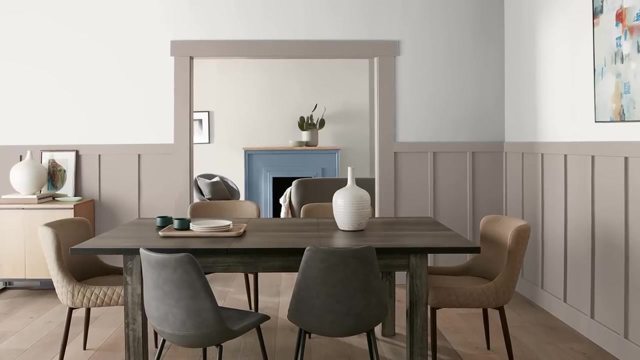 Snowbound- and Alabaster is Snowbound- has that bit of brown kind of amped up which I guess is a little bit of a red undertone compared to yellow. It feels just a touch less warm. I don't want to say cool, because I don't really see it as a cold white, even though the name might suggest. 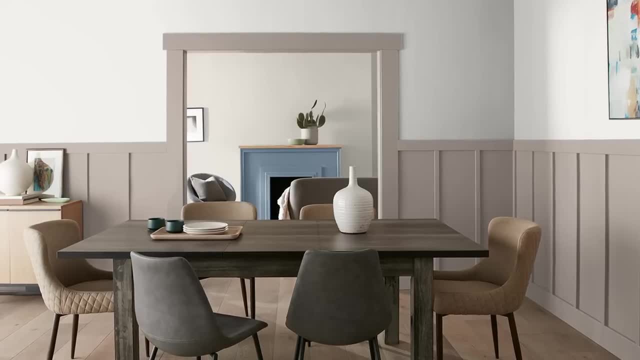 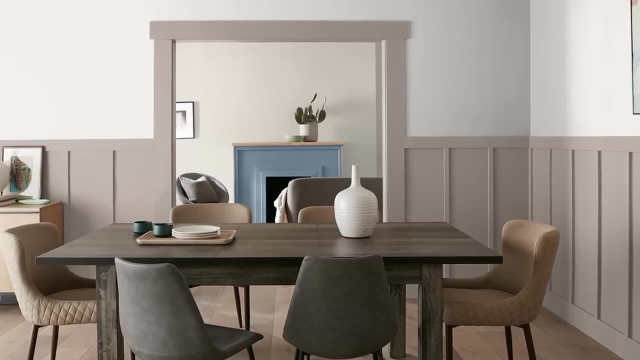 it. It's just a wonderful kind of 1A, 1B alternative to Alabaster and it's usually an easier choice if you're working with perhaps a lot of taupes and browns and reds and things like that. It might. 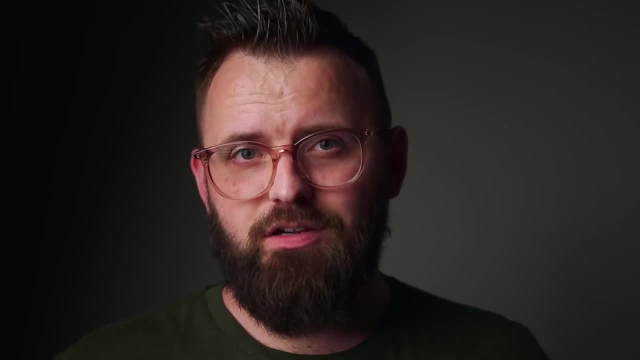 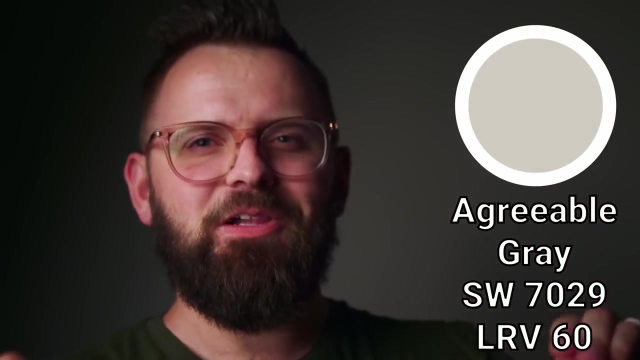 be a little bit too dark for your face, but really it is timeless, just like the rest of these colors. My third Sherwin color choice has got to be Agreeable Gray. I'm sorry, but I'm not sorry because this is a color that really bridges the gap between classic and contemporary Beigey colors. 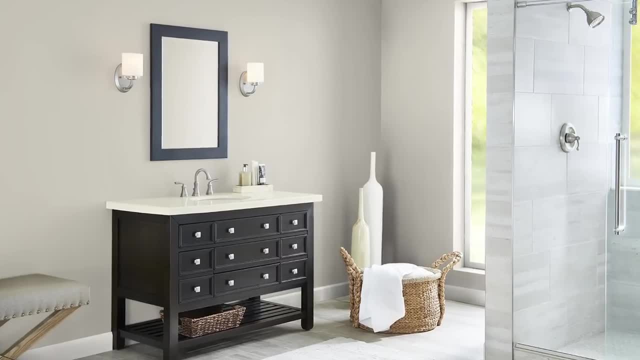 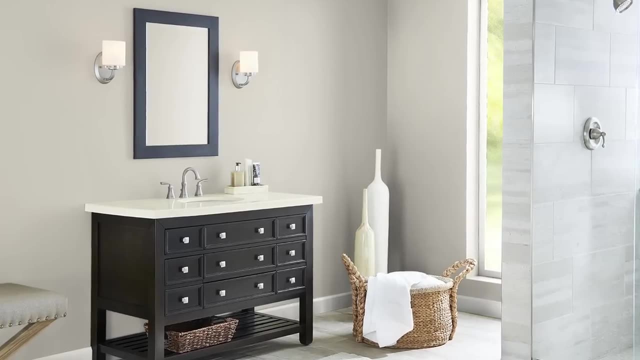 and grays. It really does that nicely. Some of you may argue that people are getting tired of this type of color because we've seen these neutrals just blow through interior design over the last decade or so. but I think it's here to stay, because 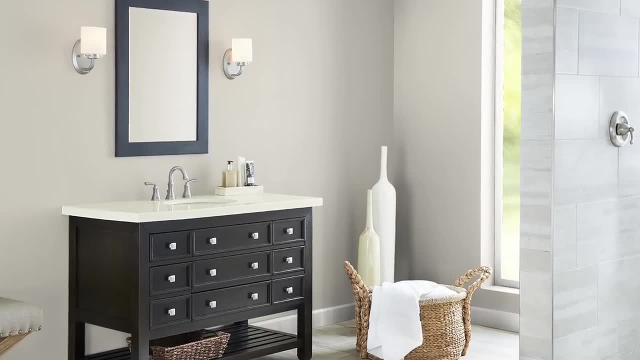 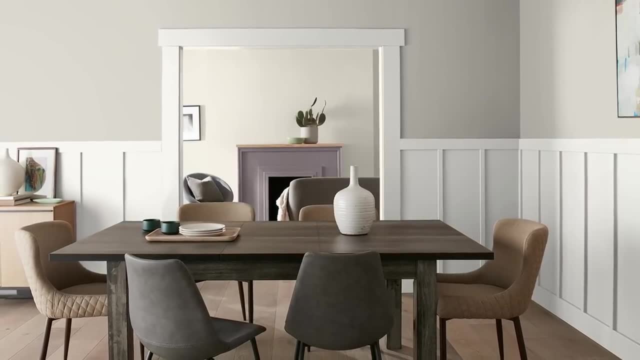 you can really put it in any situation and find a use for it. It may not be the color you would want to use throughout your home in every single circumstance. Maybe you don't want to overwhelm your space in this sort of neutrality, but there's a good chance that Agreeable Gray will work within. 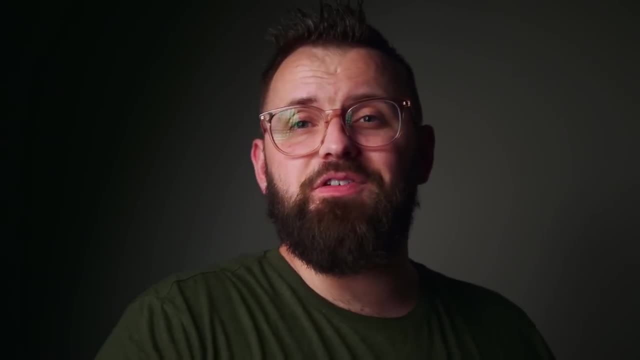 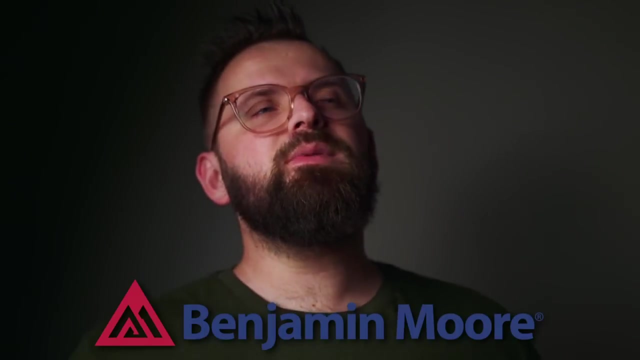 many color schemes to come. It's also nice to have a darker alternative to those off whites we talked about, because we don't all want to go light, light, light. Sometimes mid-tones are cool too. Moving on to Benjamin Moore, I wanted to lighten things up a little bit again. 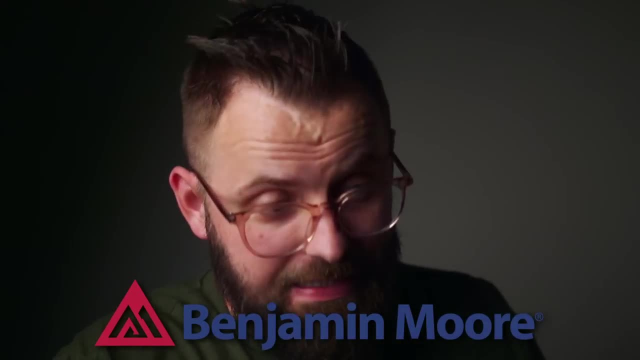 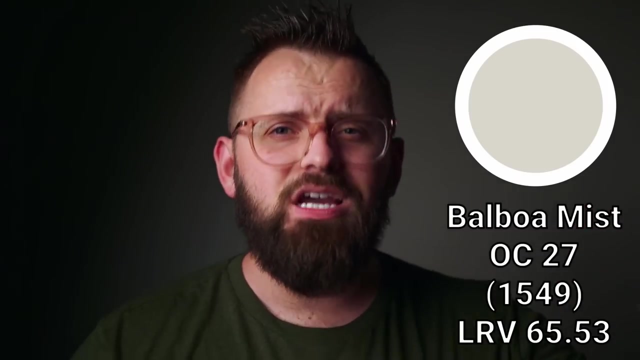 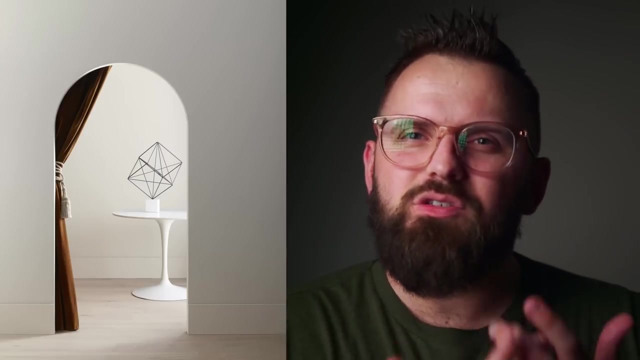 in the neutral category and present you with the almighty Balboa Mist. This is one of their best selling colors, for a very good reason. It's awesome. It's a pale grayish that is present enough to be felt, but again, won't pull focus too much either. These transitional neutrals are 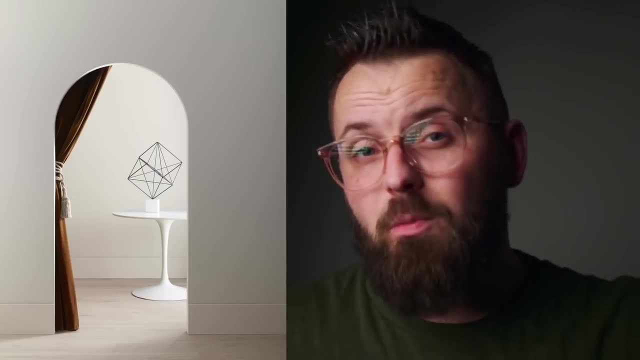 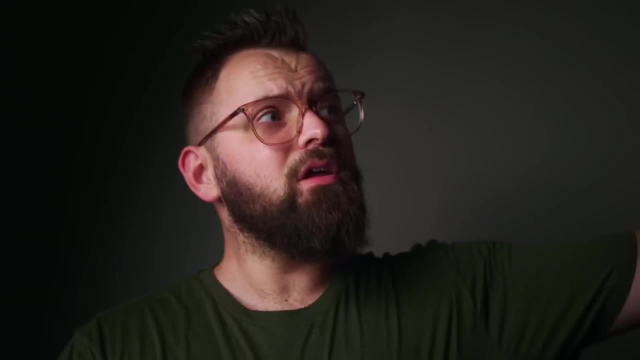 just so versatile, and as long as you're not flooding and overwhelming a space with them, I don't think you'll ever get tired of it. At least I haven't, and I've been using this color for many, many years, About as long as I've been using our next color. 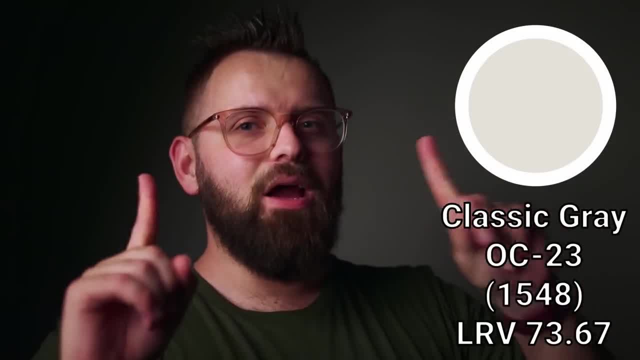 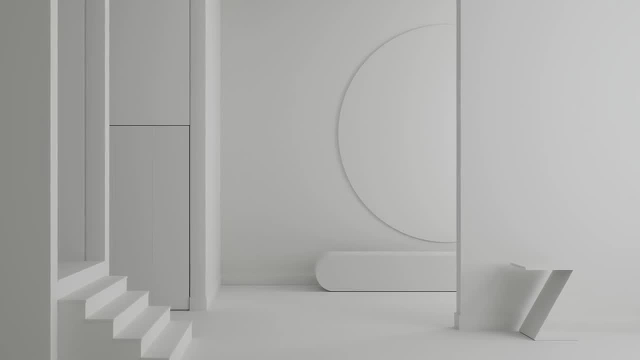 which is Classic Gray, which could be my all-time favorite off-white by Benjamin Moore. Compared to Balboa Mist, Classic Gray is a bit less saturated, a bit more gray, but it has this effortless existence that can coordinate with so many different things. It doesn't make too strong.